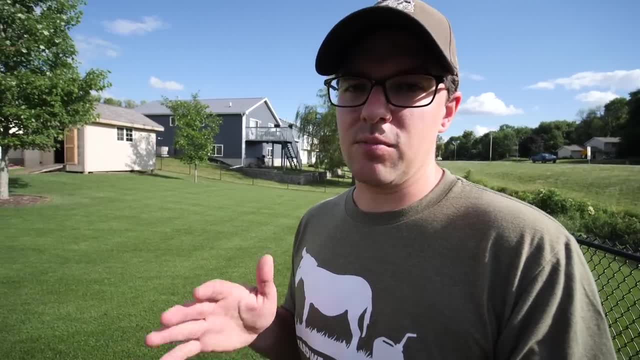 But we'll see. In cooler weather I don't usually have as much trouble getting out here and mowing it more often, But that's kind of where we're at with that. I'm going to talk about growth regulator coming up on the channel sometime. 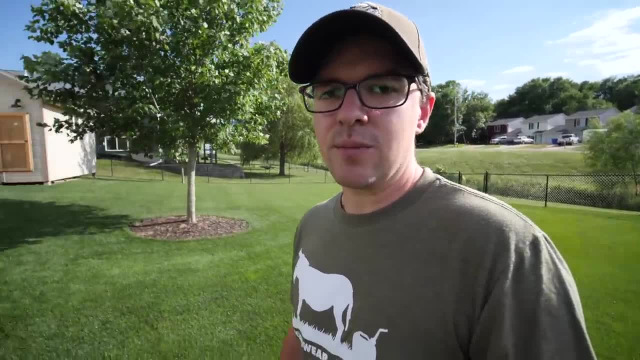 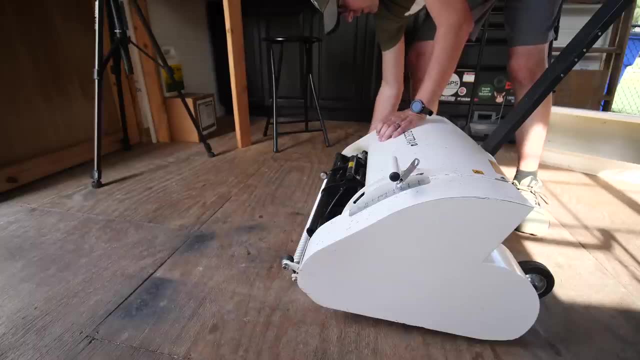 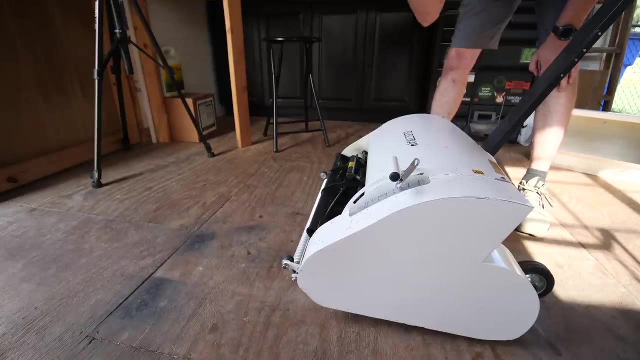 soon and kind of what you can do with that. So stay tuned for that too. Now everybody asks me why I use a certain mower at a certain time, and there's really no rhyme or reason to it. Some days I just feel like using one mower, and some days I 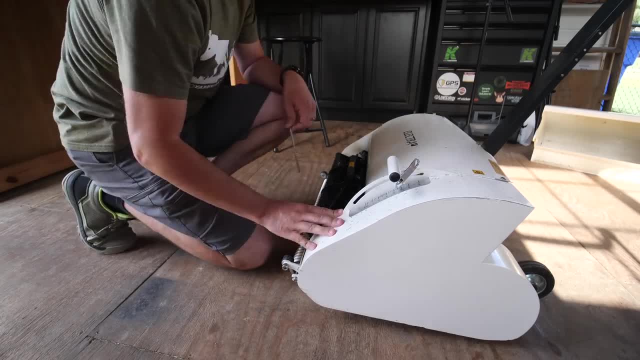 feel like using another, But with the electric mower I don't feel like using one. I don't feel like using one, but I can definitely do what I need to do with one. I like doing more work with a mower, But yeah, this is the original one and I just kind of don't have a lot more of a future. 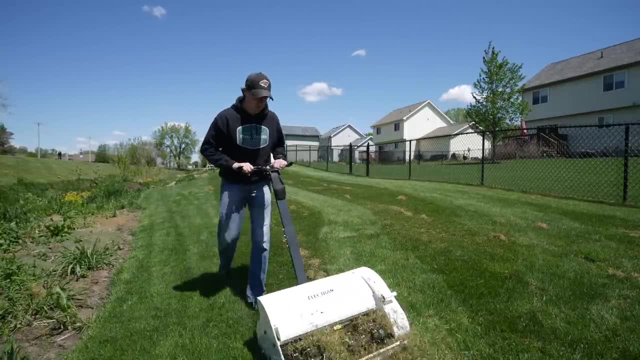 focus on this one, But for the most part I'm really just going to lean in here. I'll try to build this thing again and I'm happy to do more if it helps. So here we have the electric mower. Let's show you this. 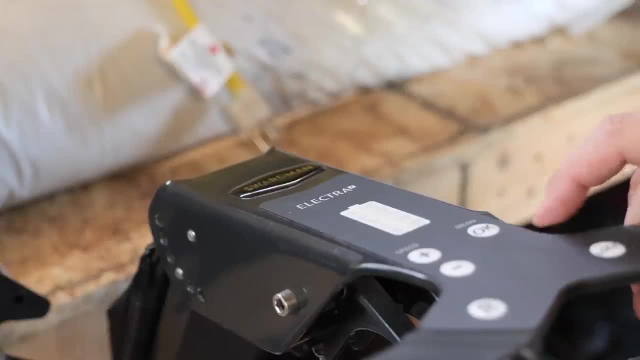 This one is a little bit different. It's a different type of mower but it has a different type of mower. The electric mower is a lot more maintained in the ona- подготов system, So you have more of a lighter feel to it. 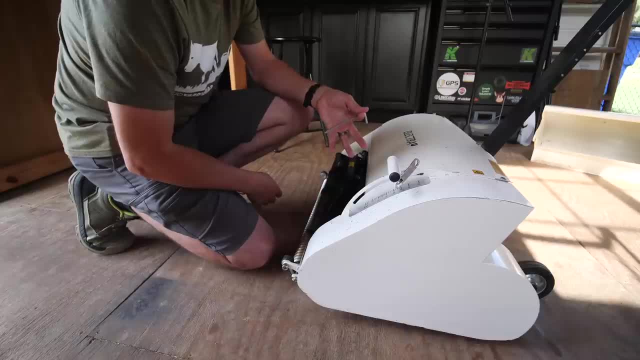 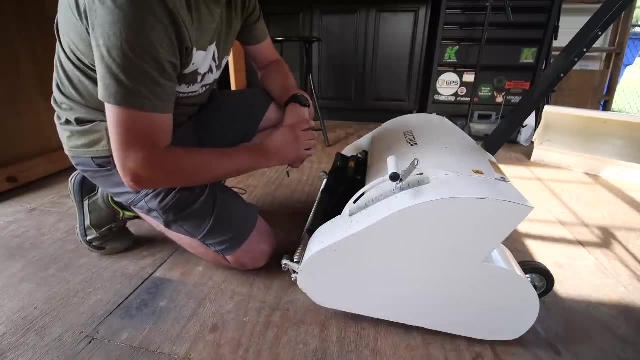 It's more predictable. You got more of a more logical feel to it, the electronics, whereas the edwin is still kind of traditionally done with a wire on the handle, pulling a belt and pulling that sort of system, and so they just feel slightly different in the 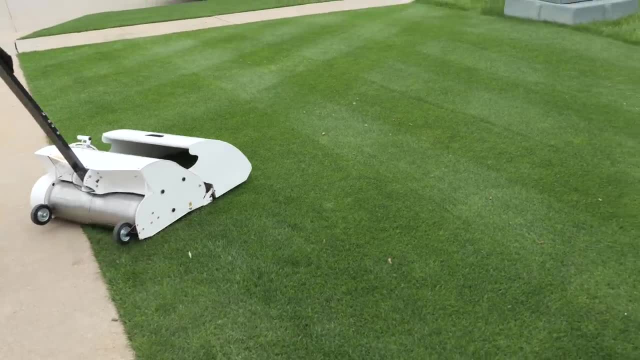 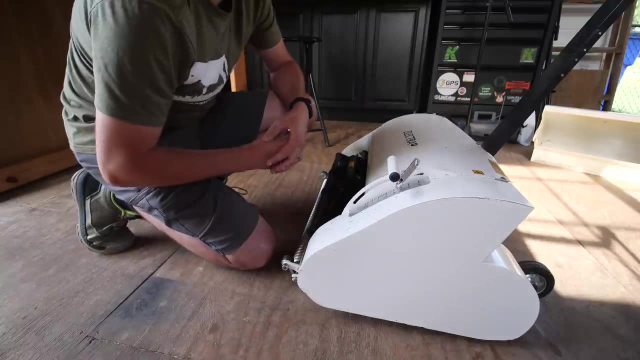 way they mow, because this one is more electronically set to speed and stuff like that and you can vary everything but you just sort of get used to whatever speed it is. there's really no way for me to describe the differences exactly in feel, but they just do feel slightly different and i just 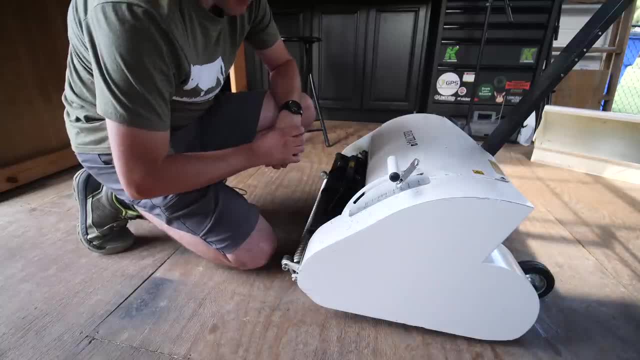 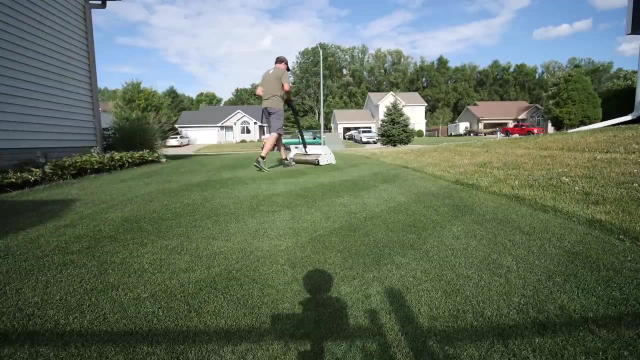 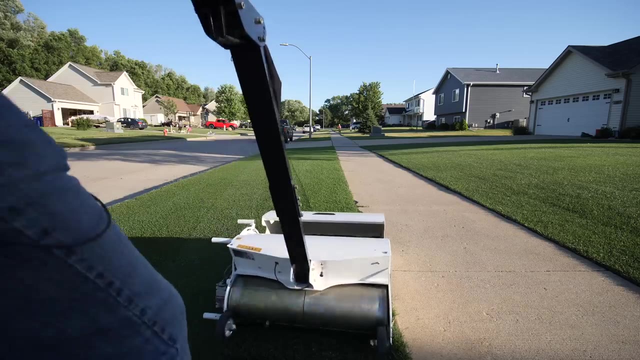 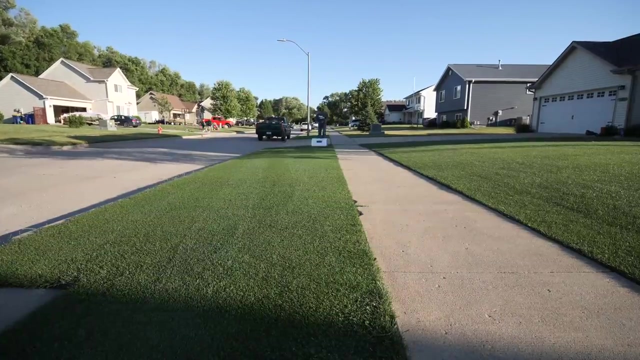 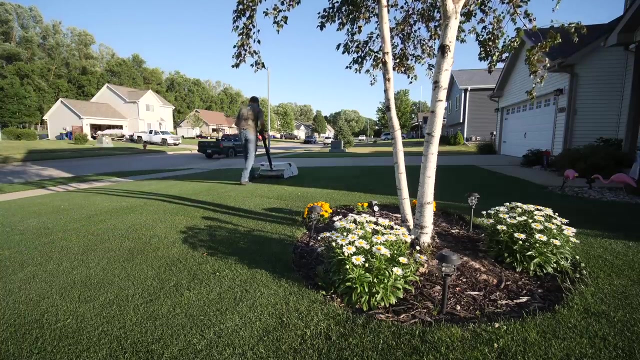 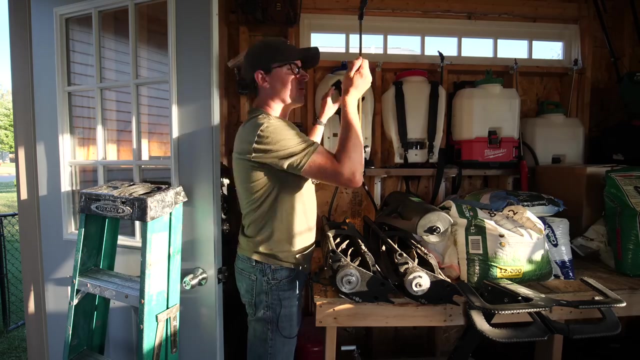 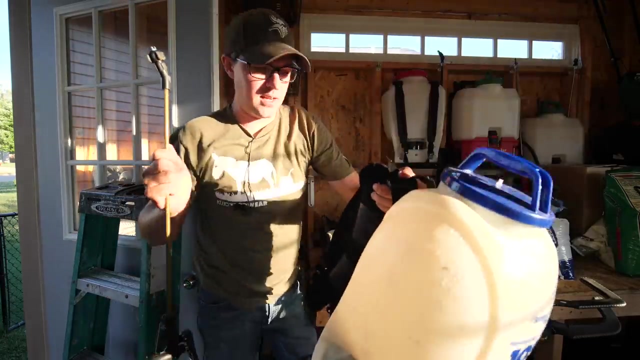 like mowing with that, edwin, and nothing wrong with mowing with this, but just my thoughts. so back to some nighttime spraying tonight. i'm doing this as often as i can when it calms down here, because trying to spray during the day is impossible and plus it's been too hot to do that. 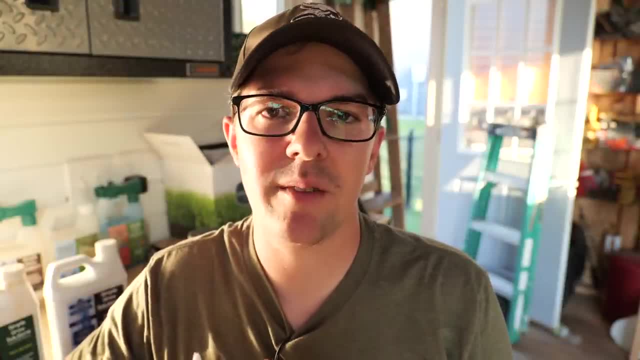 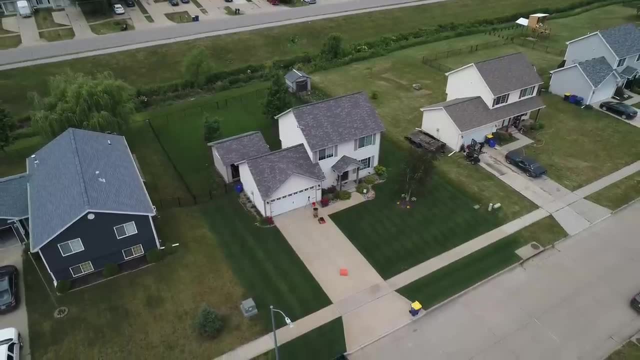 anyway, but so micronutrients were something that i kind of neglected in my program for quite a while here, and i've seen some major strides in terms of better color and, i think, overall just the health of the way that the lawn looks after i started using micronutrients. now this isn't any sort 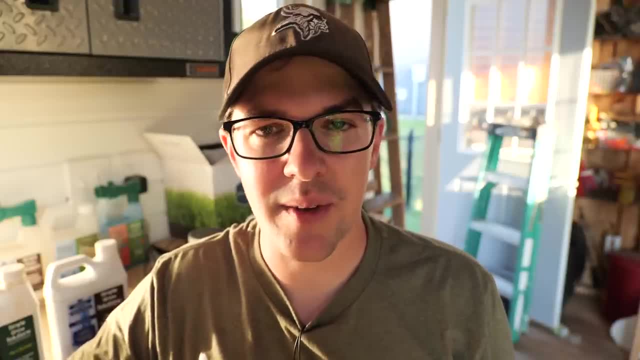 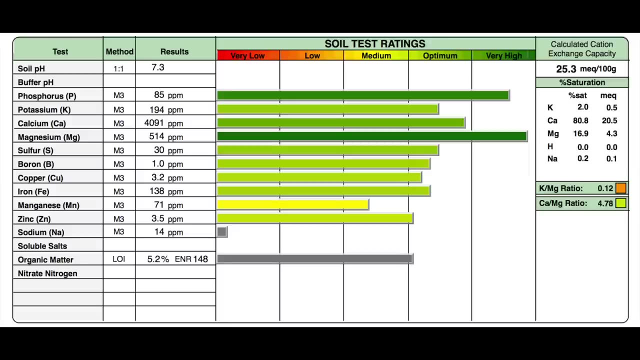 of weird thing that you're applying to the yard. you just most people talk about the macronutrients, which is nitrogen, phosphorus, potassium, and kind of forget about the other ones. especially for a ph like i have, which is higher than seven, then the iron that's in my soil is not going to be as 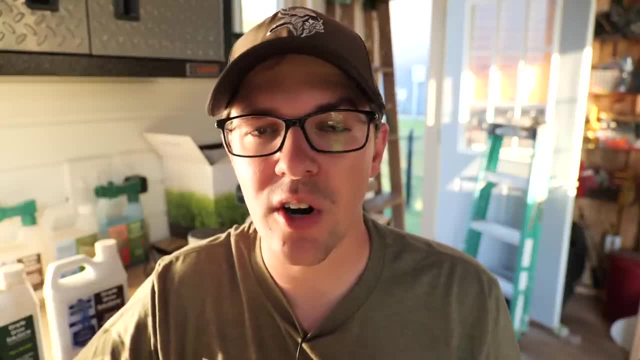 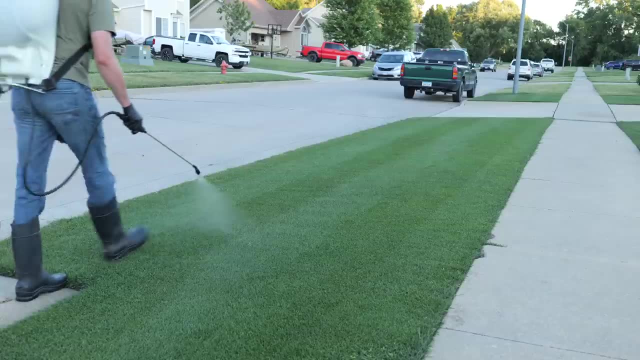 available to the plant, which means that i might struggle with getting the darker color to come out quite as much as some people who have a ph within range and also more iron available to them. so applying this iron foliar onto the grass, putting it right directly onto those leaves, has 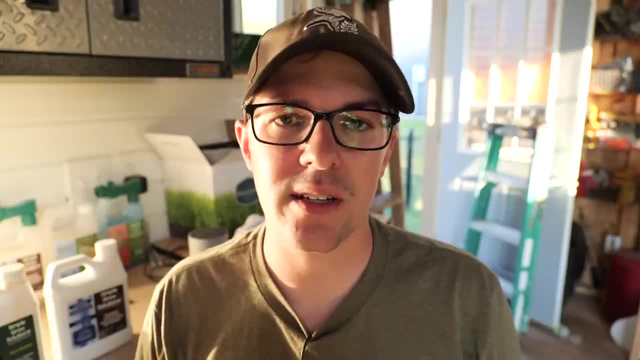 helped me a lot in terms of getting the darker color to come out. so i'm going to go ahead and apply this iron foliar onto the grass. putting it right directly onto those leaves has helped me a lot to maintain more color. maintain that darker green color that i'm going after and also the rest of 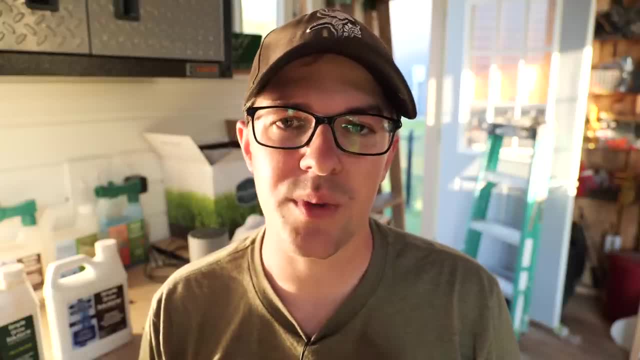 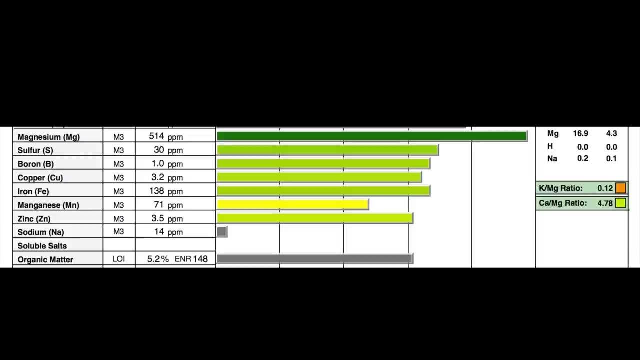 the micronutrients that are there. these are all in small doses but they're going to help the overall health of the plant, especially if you happen to have any sort of deficiencies in these and you don't need a lot of micronutrients to get back to where you need to be. but i pretty much go every. 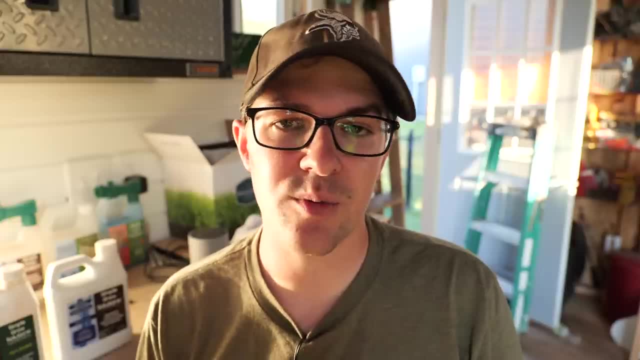 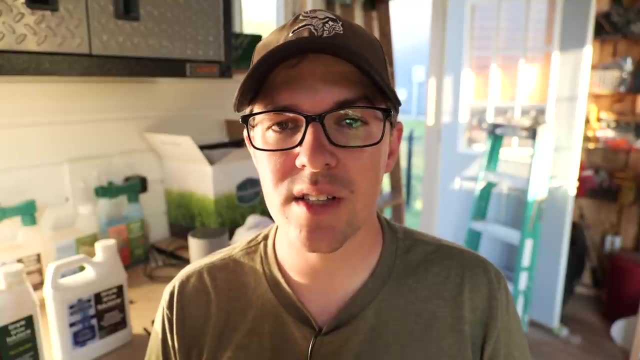 other week, with one week doing my liquid fertilizer, then the next week doing some small doses of micronutrients like this. it's been a program that's been working pretty well for me since last year. i think i've made some big strides here in terms of overall health and color. because of some 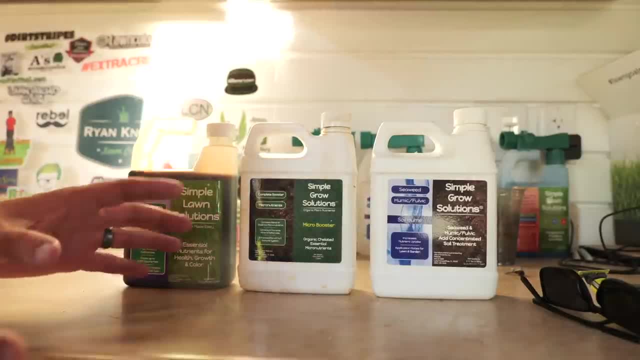 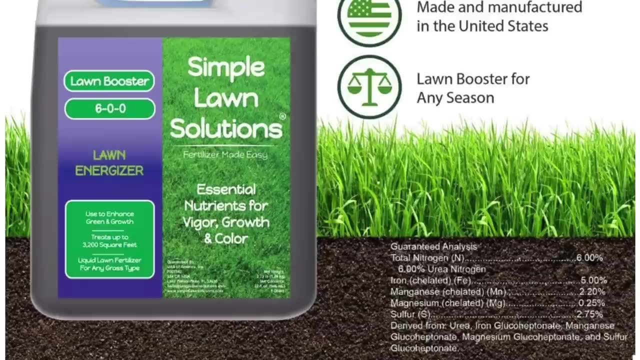 of these micronutrients that i've been focusing on. so let's look at some micronutrient options here. this is the lawn energizer which comes in my box that i have, and this is basically just a little bit of nitrogen to carry things, but mostly we're looking at iron and a few other micronutrients in. 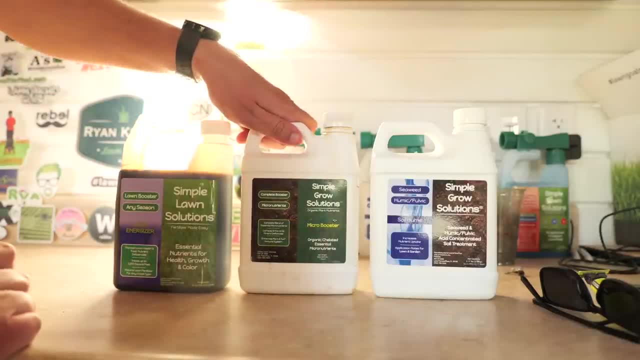 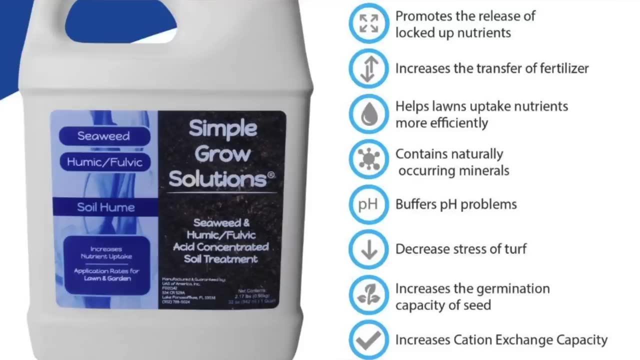 here to add. along with that, this right here is a micro booster, so it's simply focusing on the micronutrients on this side. sometimes, what i'll put in here is a little bit of, a little bit of a little bit of oxygen, and that's going to be some of the micronutrients that i want to put in here. 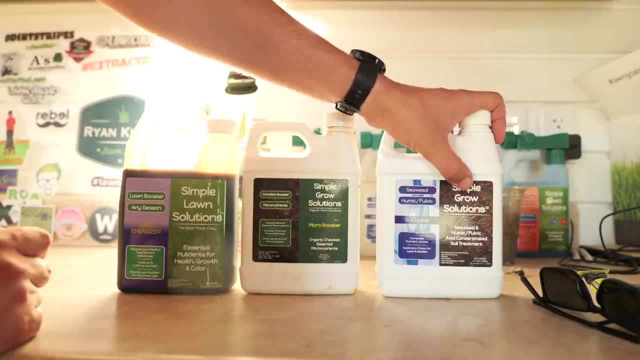 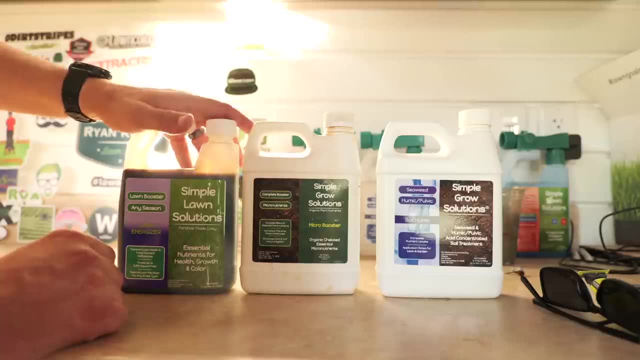 um, the first thing i put on before that is some soil hume which has some kelp in it and humic and fulvic. normally what i would do with any of these is put these down with the hosen sprayer and make sure that gets water to the soil. let some of it sit on the leaf for the fulvic acid to sit on the 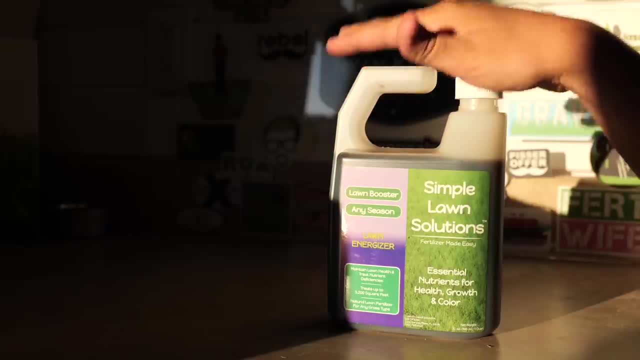 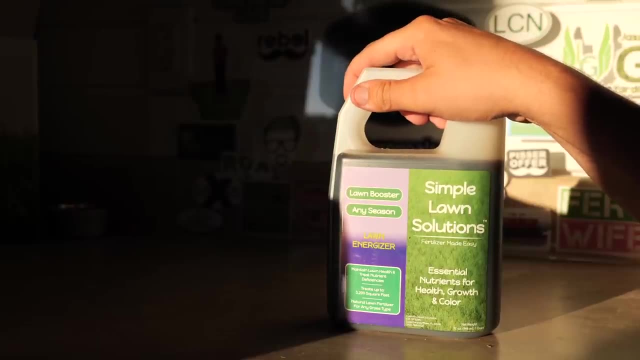 leaf, then go ahead and apply my micronutrients or either of these. and even for those of you that are on more of a granular program, if you are interested in using some kind of liquids during the summertime, long as things aren't dormant, then you can use something like this. It does come in bigger bottles. 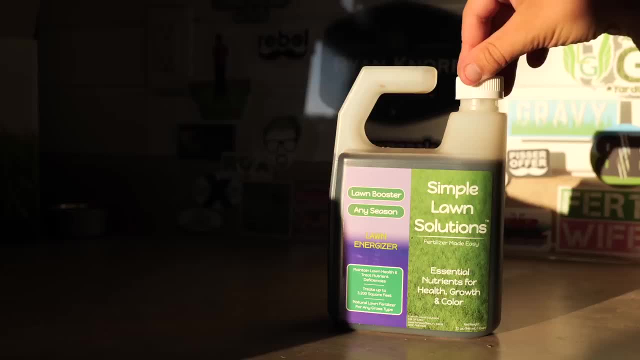 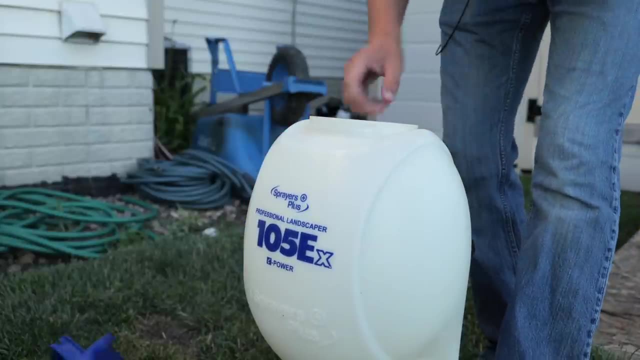 too, and also comes with the hose end sprayer, if you would like to just attach and spray this out. As I've mentioned before, I just prefer spraying with the backpack for things that I want to do fuller, because I just want it to sit more on the leaf if possible. So I'm going to fill this thing. 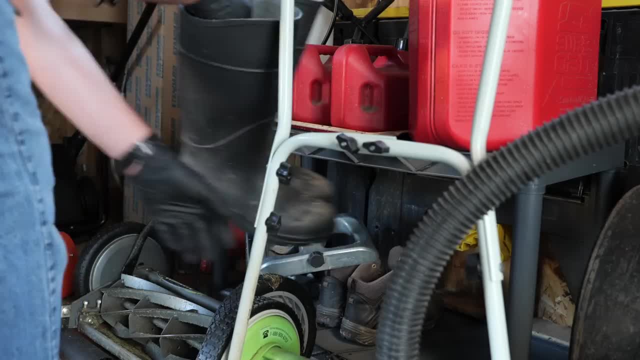 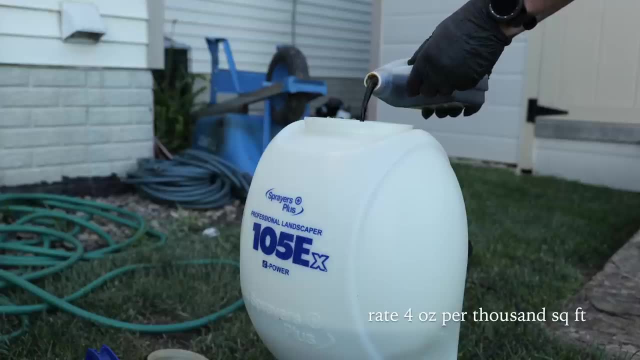 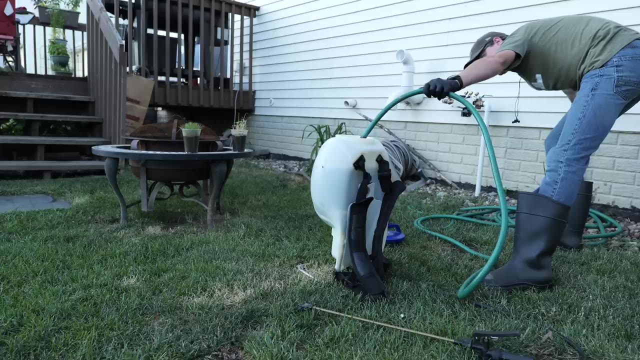 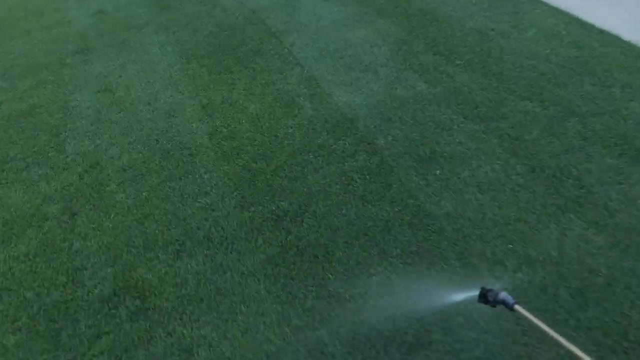 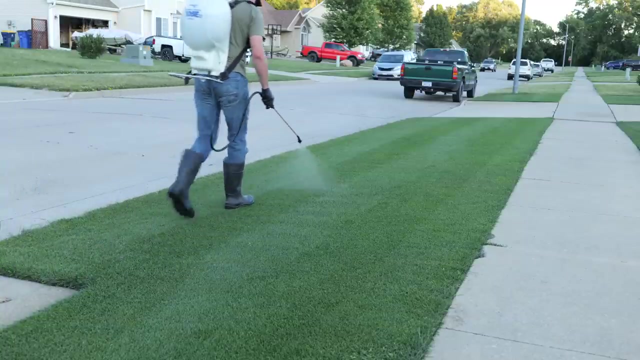 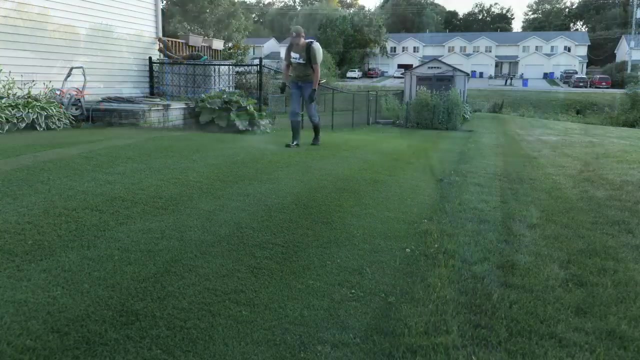 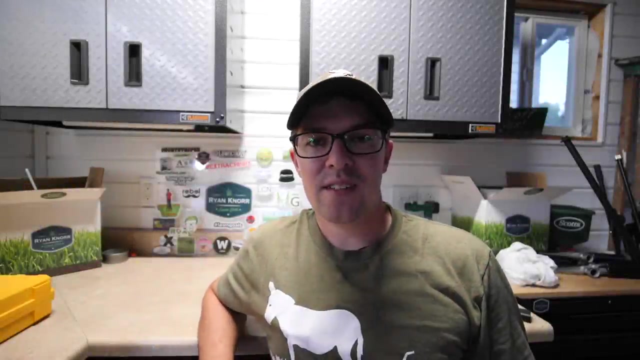 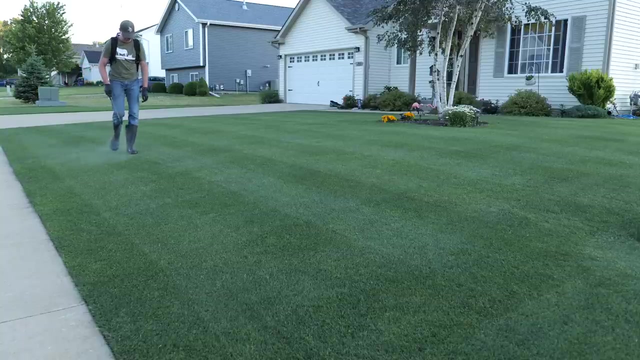 up and go spray some front yard and some side yard. So all right, so I'm going to let that sit on the leaf blades of the grass here for probably four to six hours. So I'm going to do that and actually just let this sit on there, soak in and then water that. 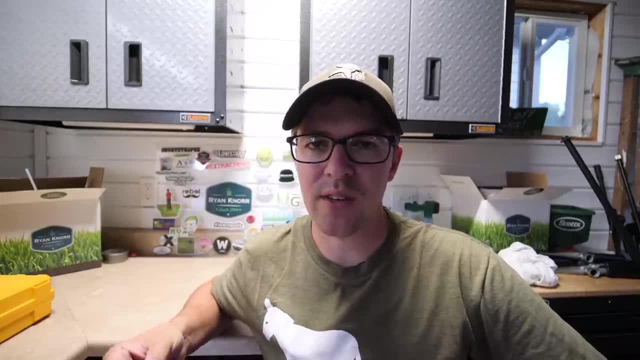 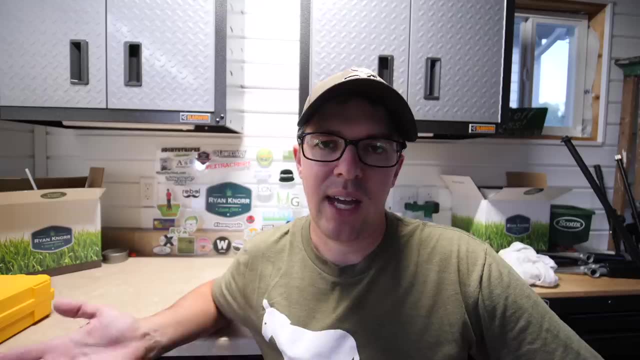 in in the morning. You also might notice that some of the actual leaf blades of the grass in the morning might have a sort of a brownish tinge to them because the color of the material and the iron actually spraying on there and sitting on the leaf and if you water this in it should minimize. 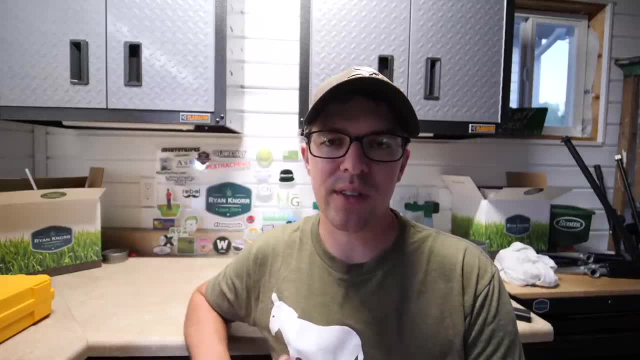 all of that stuff too. That's really why I apply my micronutrients, especially the iron, to give me a darker green color. So check out some more videos here on the channel. Thank you so much for watching. We'll see you next time.